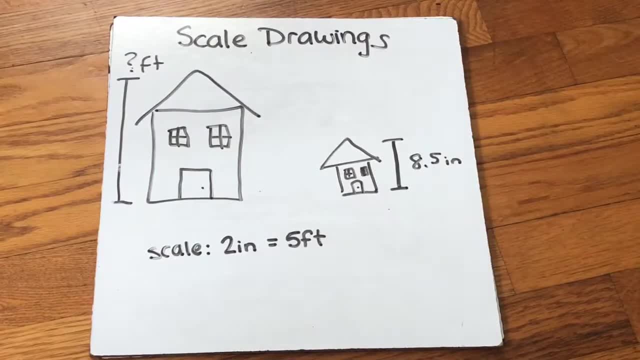 Let's do an example of scale drawings. Scale drawings are part of proportional relationships and scale drawings are used when we are trying to draw something that in real life is much too big to draw to actual size, So the scale of it's too big. we need to shrink the scale down to something so we can. 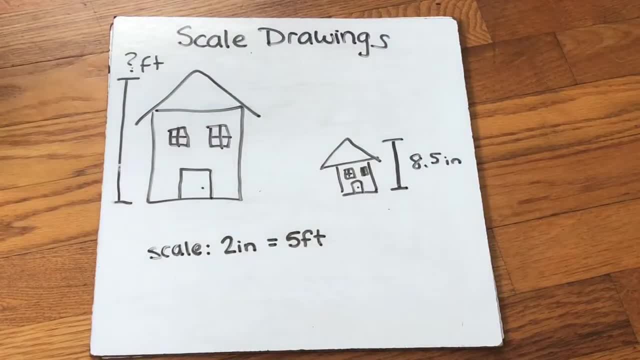 actually work with it. So the most common way we see this is in architecture. When somebody's planning a building to build a house, to build a mall, anything like that, they're not gonna find a massive piece of paper and roll it out over. 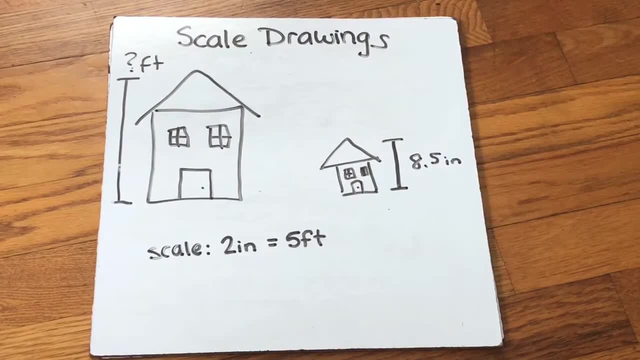 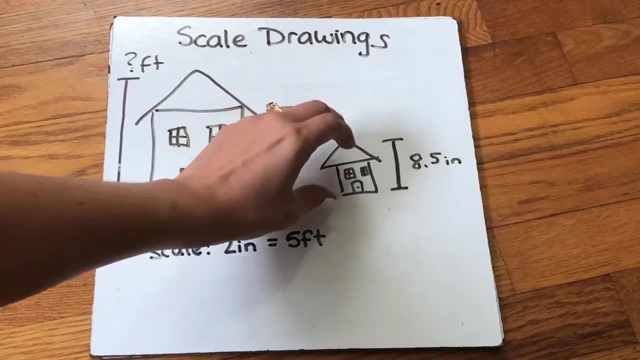 football fields and try to draw it to the actual size that it is. That would be crazy. What they're gonna do is they're gonna shrink it down to a smaller scale so they can plan it, and then they'll know what their scale is will equal what. 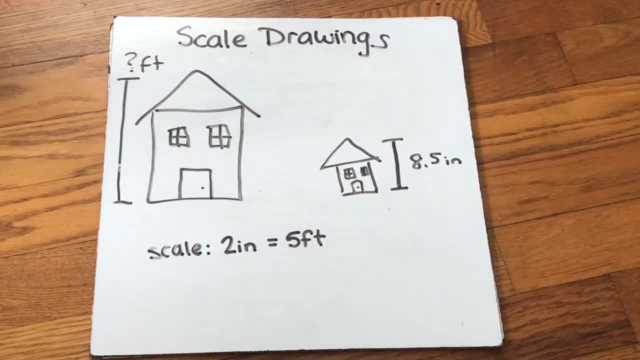 it's gonna be when it's bigger. This needs to be really precise and accurate so that your windows fit and your doors fit and your stairs go in the right way. So these numbers really need to be precise, So the scale needs to make sure. 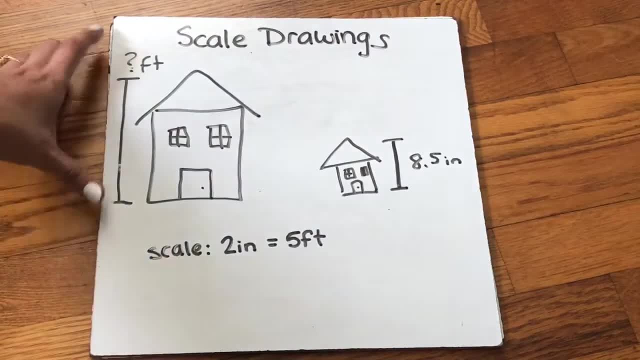 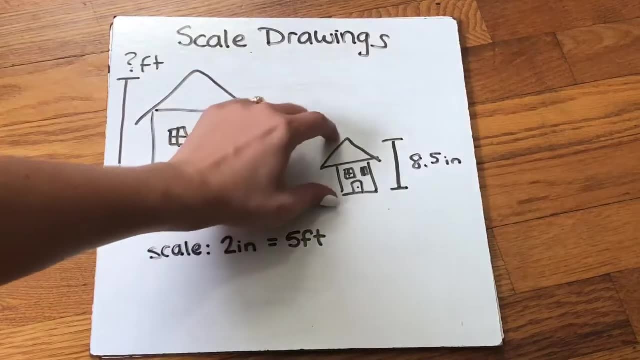 it's the same. So let's look at this problem that we have. Here's my regular sized house. This is the big house and it's a certain number of feet, but we don't know how many feet it is, But we know that the little drawing that they did of it is. 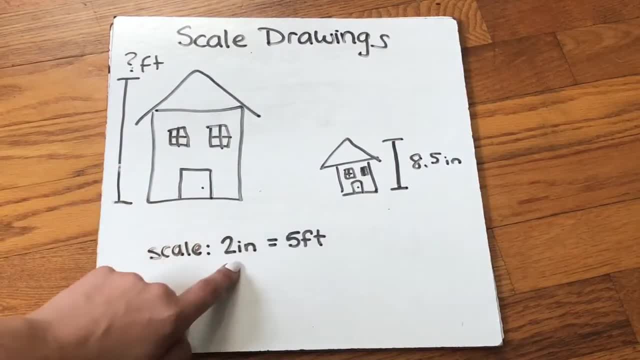 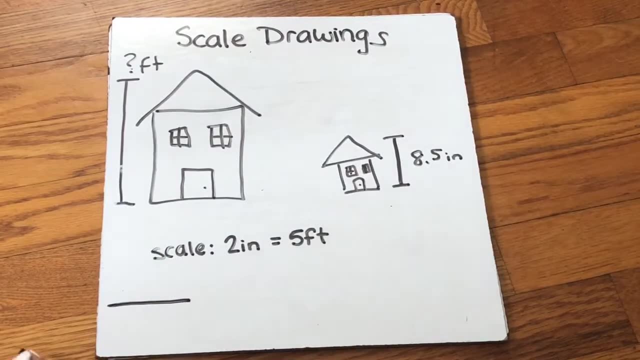 8.5 inches and we are told that our scale is for every two inches it's five feet. So when I set up a proportion, first I draw my words. So I have my words contain my units of measurement. So in this problem I have inches and I'm 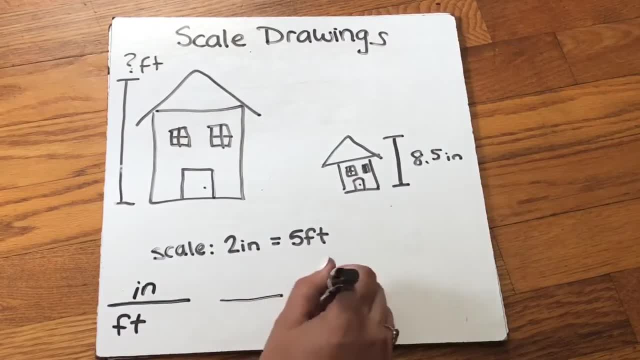 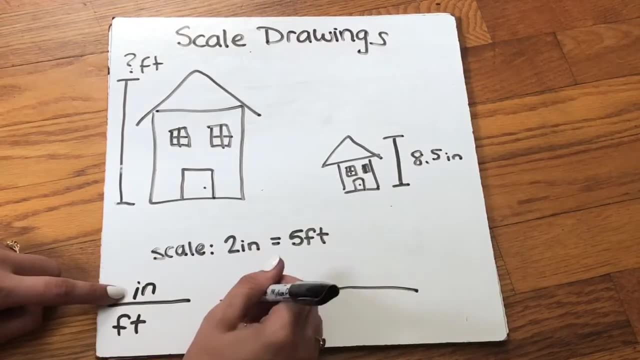 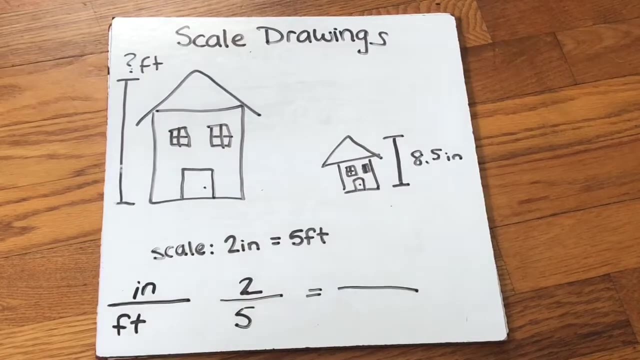 comparing those inches to feet. So now I'm going to draw my skeleton and my scale is two inches to five feet, So I'm gonna make sure two lines up with inches and five lines up with feet. making sure everything is matching is really important in all proportional relationship problems. 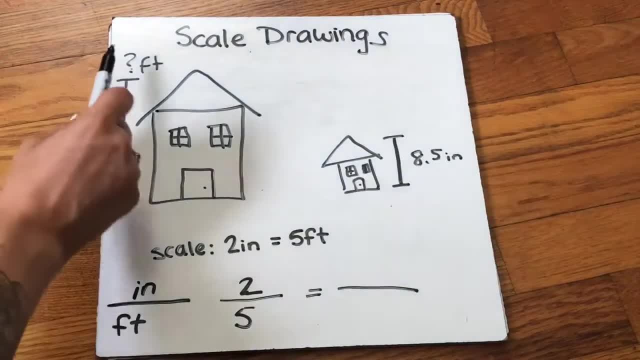 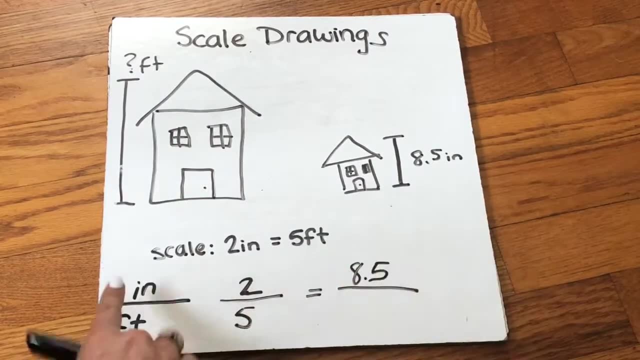 Alright, now I'm gonna look at what my problem gave me. okay, We're looking for feet. we don't know feet yet, but they gave us eight point five inches, so I'm gonna line that up with inches. and now I'm gonna do my fish or cross my. 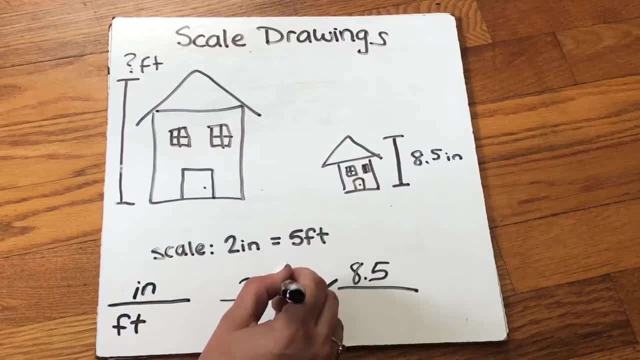 multiply and divide them. Do 8.5 times 5. divided by 2 equals, and that equals 21.25.. So what does that mean? So that means that if my scale is for every two inches, you have five feet in real life.